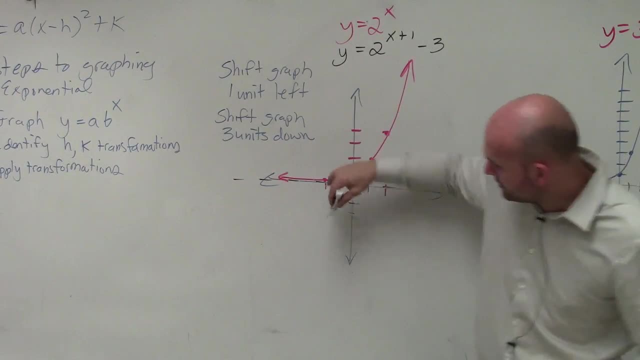 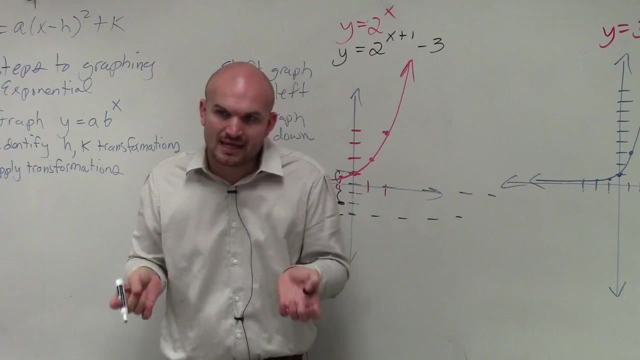 at zero and I go down one, two, three, So now I create this horizontal asymptote. What's what the point? the reason why it's important to have that horizontal asymptote is because this graph, as you guys can see, approaches the asymptote at zero, right? 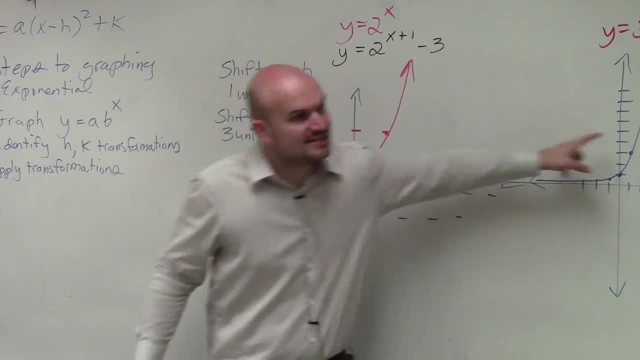 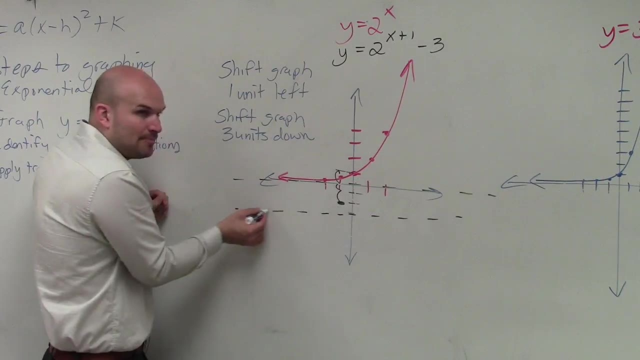 Remember we talked about it does not cross Jasmine, It does not cross zero. It keeps on approaching this asymptote, right? So, in the same respect, this graph is going to keep on approaching this asymptote. It's never going to intersect the asymptote. 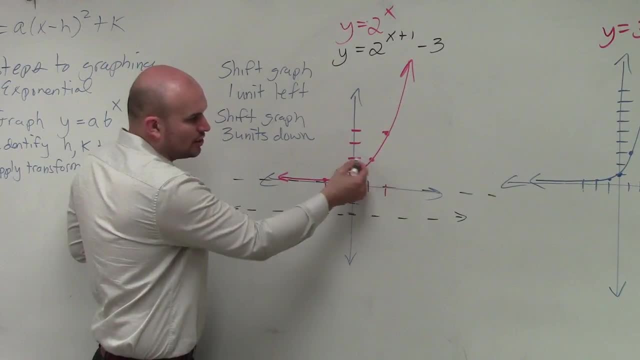 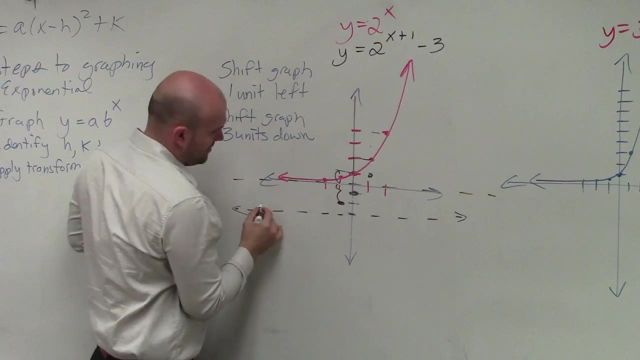 So now all I'm simply going to do is take all my points, go over one down three, Over one down three, And you guys can see. my graph is now with the transformations in the black. Yes, George, The one unit left, but isn't it one with a positive? 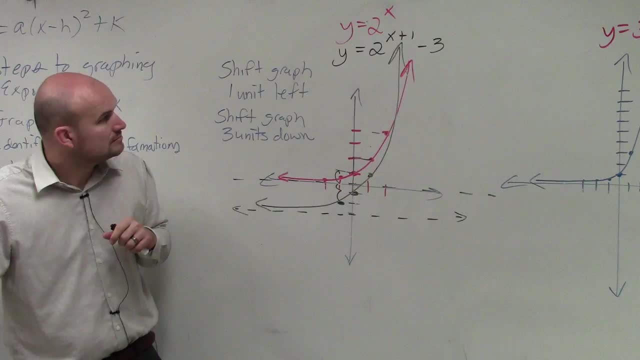 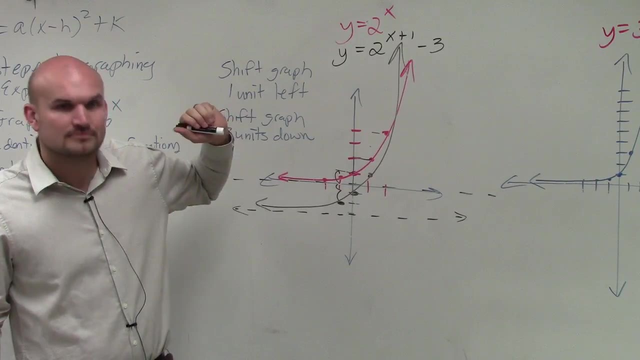 I'm sorry. The one unit left, isn't it positive one? Should we go to the right? This one, Yeah, Yeah, so you've got to go to the left. It's always the opposite. Oh, okay, Okay. 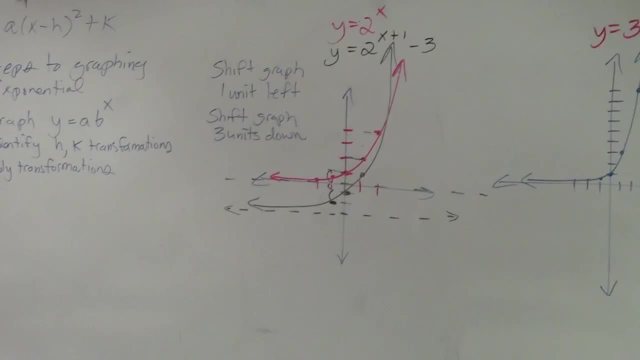 Do you make sure that makes sense? 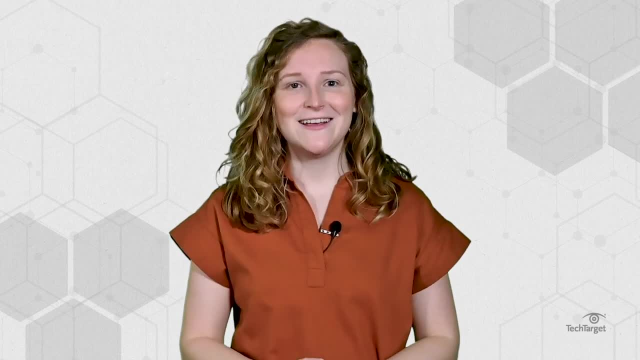 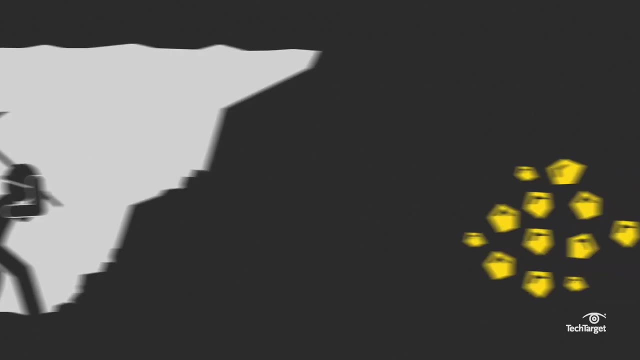 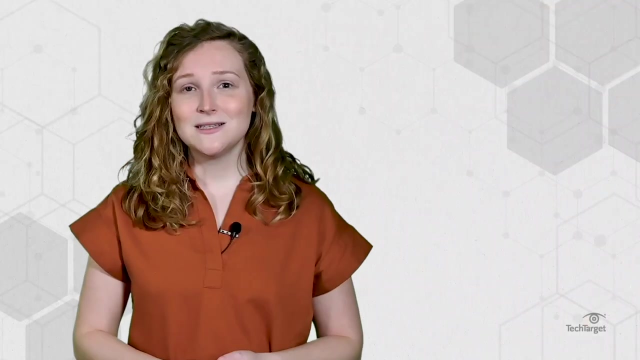 Looking for gold in a mine of information, Data mining can help. Like how mining for gold is digging through earth and rock for the valuable bits, data mining is sorting through large data sets to find the valuable information. The process of data mining involves using software, algorithms and statistical methods.